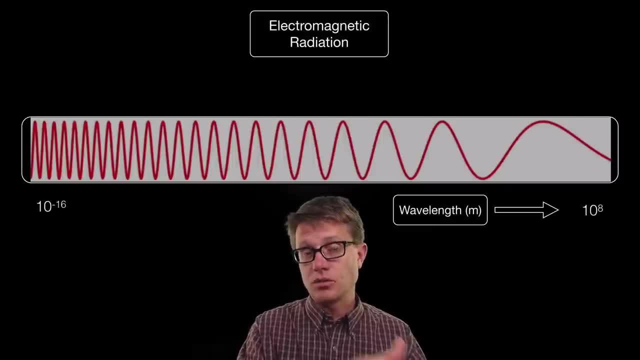 it on a spectrum and measure it from the really low, small wavelength to really long wavelengths, up to kilometers in wavelength, And then on the other direction we are going to have increasing frequency. So as we increase frequency we are going to decrease that wavelength As 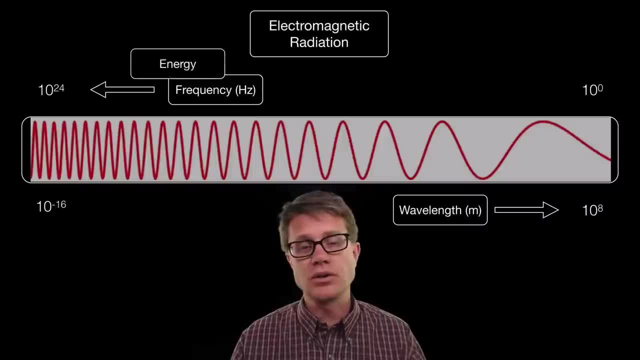 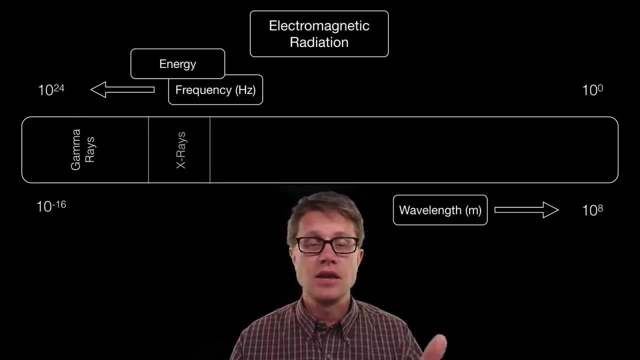 we increase frequency in electromagnetic radiation, we are also increasing the amount of energy, The energy that those waves have, And so if we start with really high energy, we would have gamma rays, then x-rays, then infrared and then visible light. So you can see that. 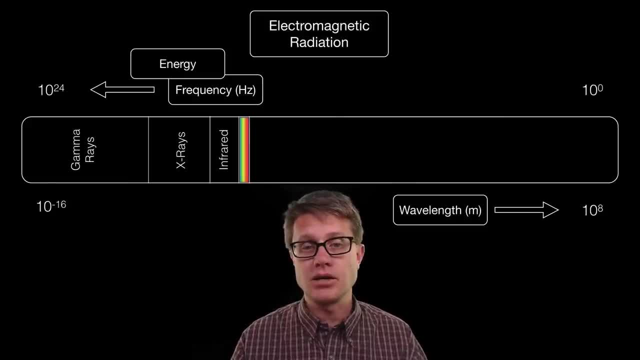 we are just seeing a small sliver of electromagnetic radiation. We then move into ultraviolet, finally into microwaves and radio waves, And so inside this room right now I have visible light, But there are also radio waves here. That is how you could pick up a radio signal, or? 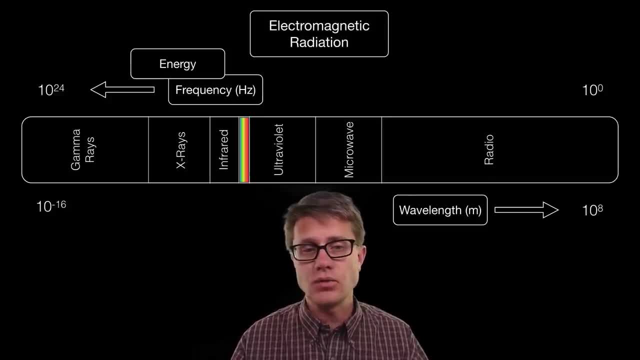 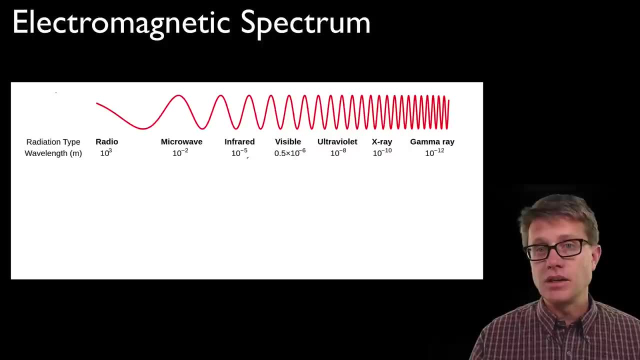 a TV signal, But I also probably have microwaves in here as well. Hopefully I do not have too many gamma rays in here right now, But if we put them along a spectrum they are going to decrease in wavelength as we move towards those gamma rays. To give you a sense of scale: 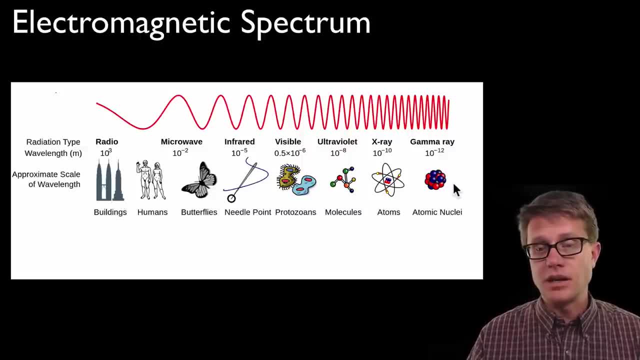 radio waves are going to have wavelengths around the size of a building, But gamma rays down around the size of a nuclei, And there is this inverse relationship. So as we increase wavelength we are going to decrease the amount of frequency, And so as we increase frequency, 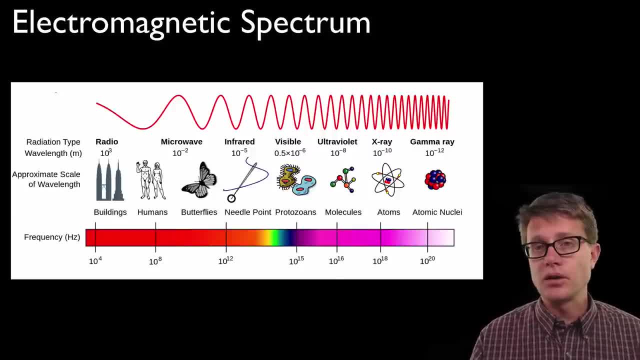 we have higher amounts of energy, So which one would you rather be expecting to have exposed to These ones? with long wavelength, really really low frequency, low energy, The ones on the right side are going to be able to damage cells, ionize cells, cause. 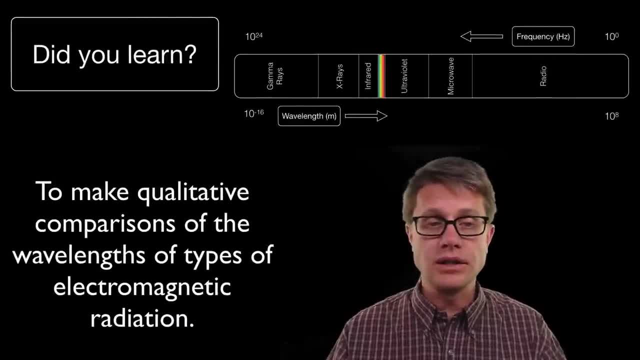 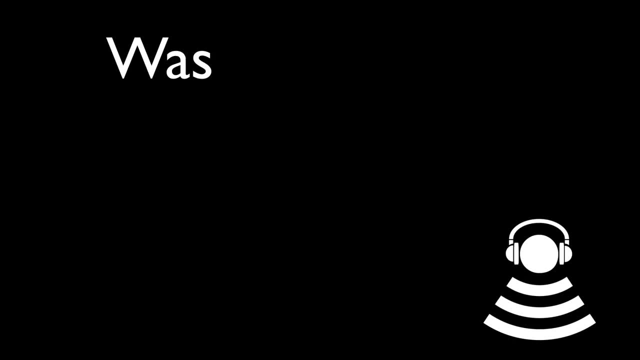 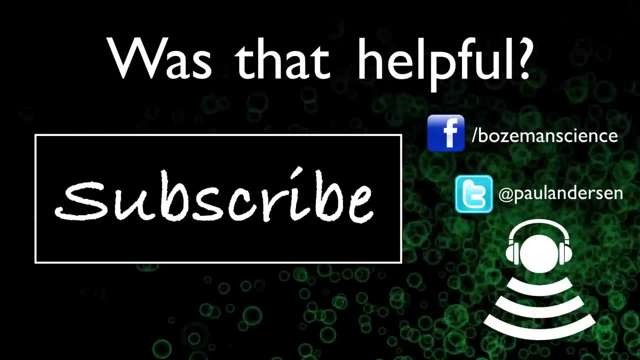 damage to the cells itself, And so did you learn to just make qualitative comparisons based on wavelength and frequency of electromagnetic radiation? I hope so, And I hope that was helpful. Thank you very much.